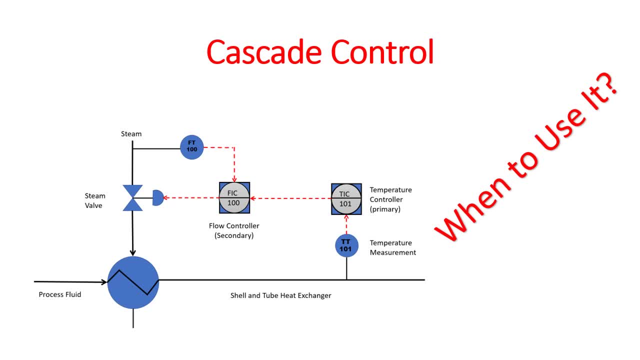 or this configurations. So we will be discussing all about this thing. So this will be Through and through understanding about the cascade control and once you complete this lesson, I'm sure you will be very much confident about the cascade control and you will be able to answer the interview questions, or you will be more confident in implementing. 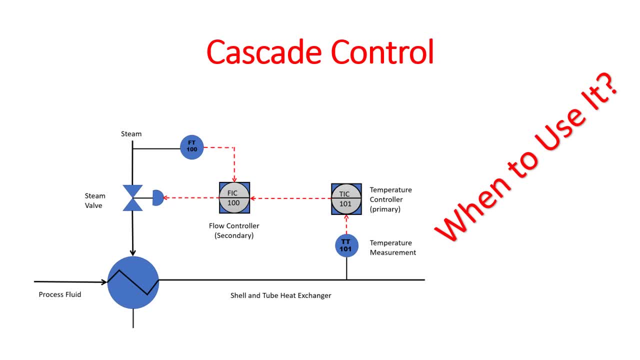 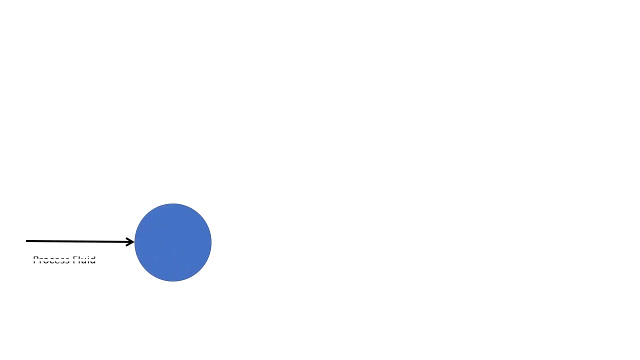 the cascade control, either during the project phase or if you are in maintenance, tuning the control loop or the troubleshooting this cascade control loop, you will be very much confident. Okay, so let's begin our class. So, as we begin into the cascade control system we will be discussing about, with the help 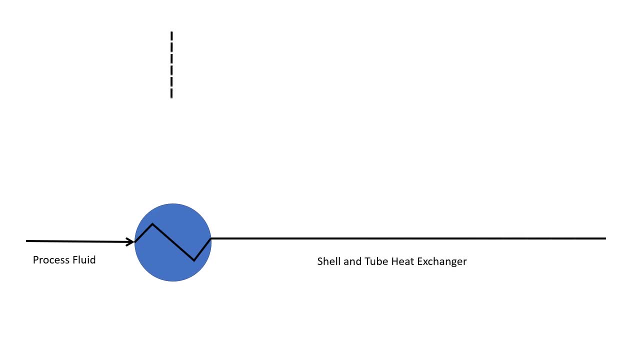 of a practical example, because- because this will give you a more detailed understanding- and this, the loop I am going to discuss, is one of the most common loop in the process industry. This loop is used in the heat refinery, petrochemical, paper industry, chemical industry. 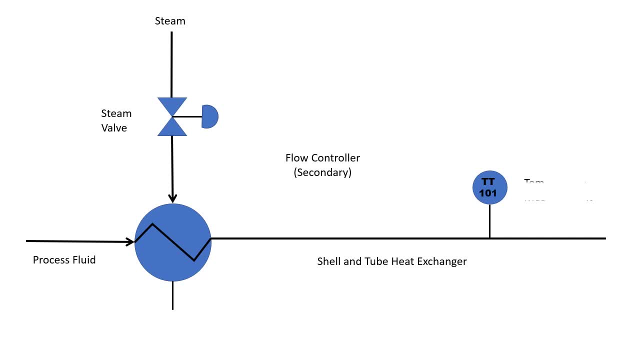 So everywhere this particular loop is often used. and yeah, so the first thing is, like it is a heat exchanger, right, and if the process fluid is going through the heat exchanger and it is being heated with the help of a steam, right, so so this is the process fluid that 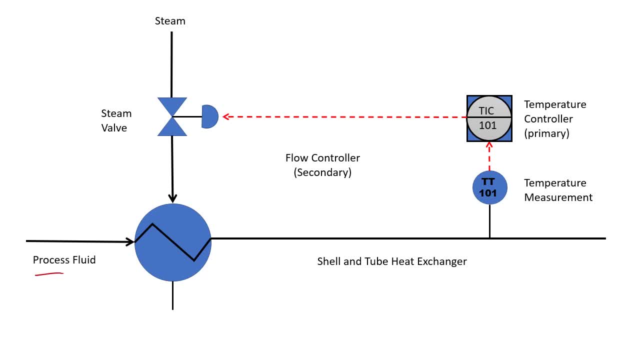 is going through the exchanger. Okay, So this is a sail and tube type exchanger, So the process fluid is going through it and it is being heated with the help of a steam. Now we want to control the outlet temperature, necessarily, because the process fluid may. 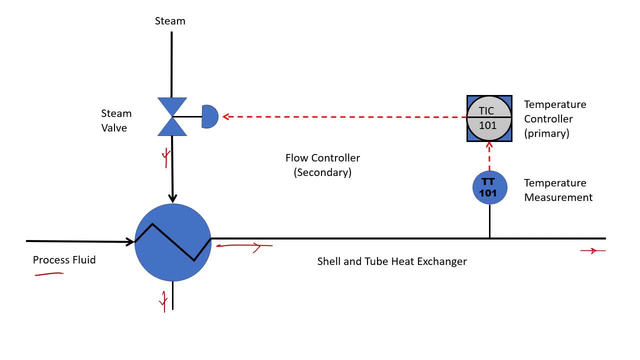 be used in downstream, in some other places, and we want to control the temperature. So how to control the temperature? So we need to have a sensor, which which will measure the temperature. Then we will have a temperature. So this temperature controller will take the input from the sensor and the operator will. 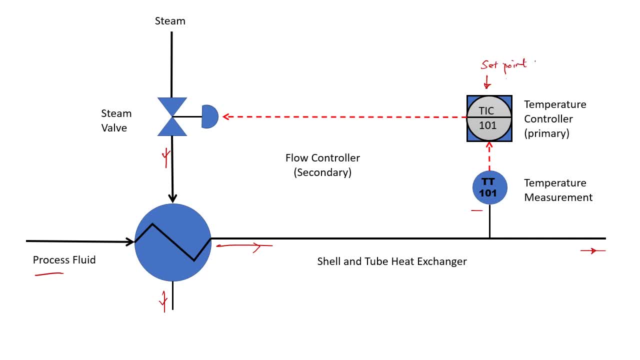 give it a set point. So at what temperature you want to control it. So say, 100 degree, or you want to control it at 150 degree centigrade. So this is the set point that the operator will provide and based on the sensor input. 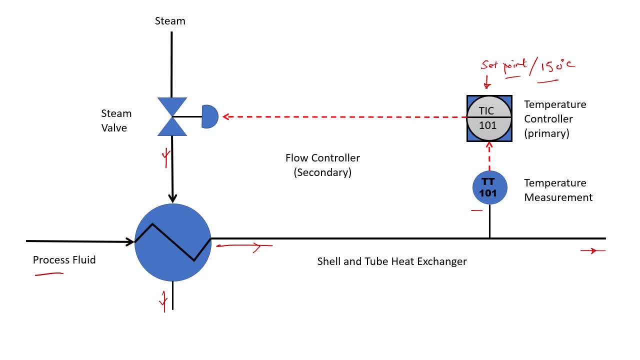 and the set point, whatever error is there, so that error gets multiplied with the PID control scheme or whatever algorithm that is inbuilt within the controller, generates an output which is called a manipulated variable, and that MB goes into the valve, the steam valve, and steam valve opening increases or decreases based on this input and as the steam 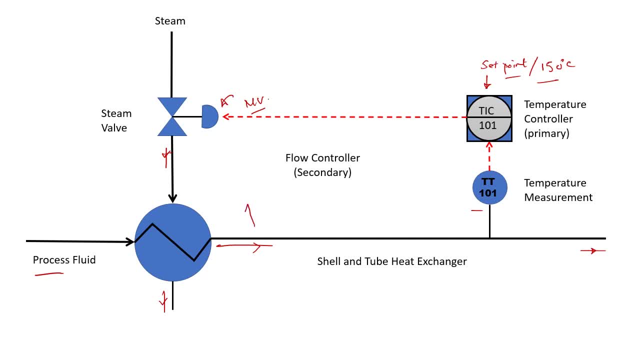 flow increases, the process fluid temperature increases. as the steam flow decreases, the process fluid temperature decreases. So this is a normal feedback control loop. So what is the issue in it? So there, there can be multiple issues. So one of the issue that common living faced is the flow of the steam is not always, I would 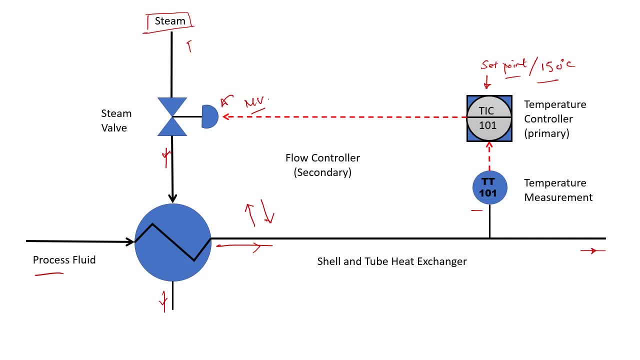 say It's fixed or there are certain disturbances. that happens in this steam line, because the steam line is basically this is an header, right, and there are multiple other things that are connected to into the header. So maybe it is connected to a turbo compressor and the compressor trips or something. any 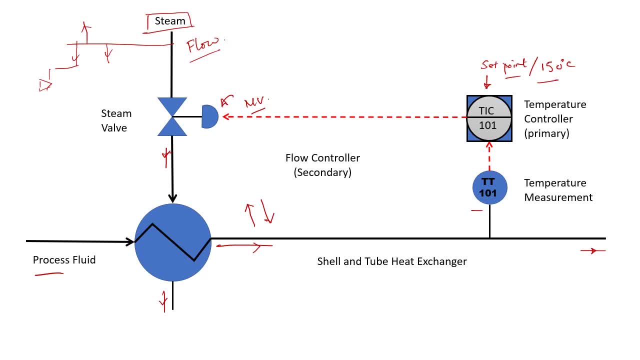 other thing happens in the upstream of the steam line And that's That's changes the flow. So as the flow, or or you say, the pressure, changes, right, So as it changes, it impacts the that. So if it, like, the valve is 30% open earlier, if you, you, there are like 10 GPM flow was. 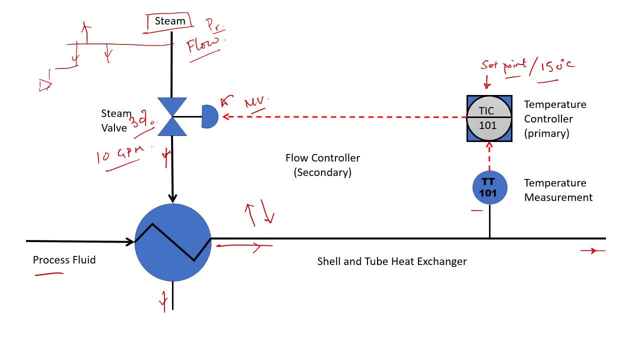 going. now, due to the upstream disturbances, the flow increases To 15 GPM right. So as the flow increases, it will obviously increase the temperature and the temperature sensor will note it and the temperature control will act on it and eventually this mb will change. 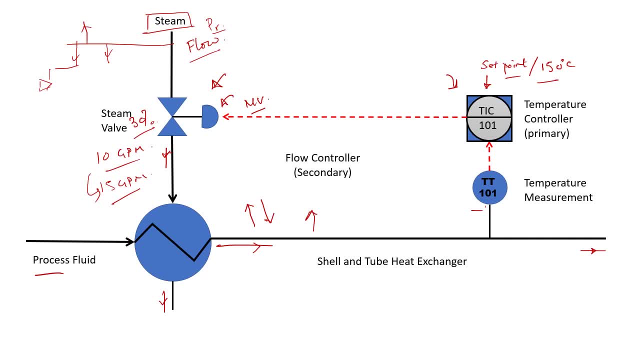 But the problem with this is this process will take a sufficient time because first, immediately, due to the increase of the steam, The temperature sensor will note it steam, the temperature will not increase, even if the temperature increases. temperature first increases at inside the heat exchanger, i would say then at the outlet, and the temperature sensor may. 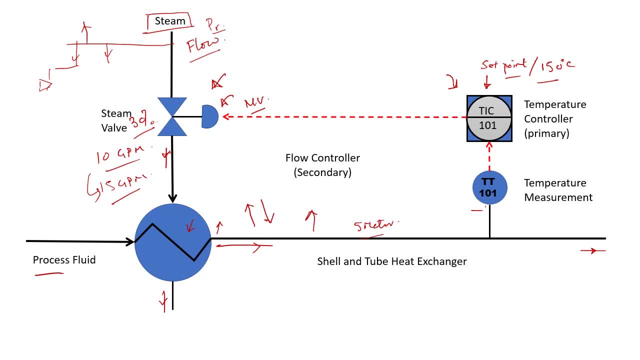 be like five meters away from the exchanger, and to increase the temperature at this point takes some more time. right, and then the controller have to act on the error and then it need to change the mb and this stream flow will then change and this process will take so much time. 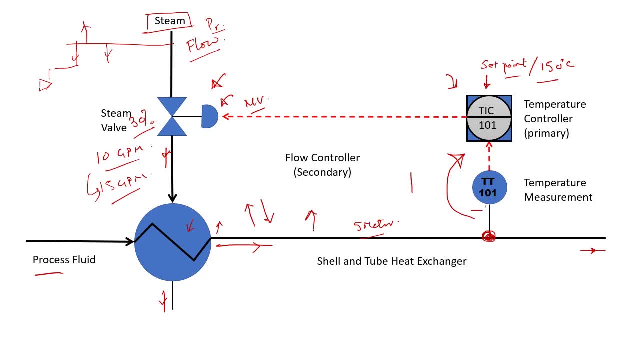 that, by the time the controller takes action, the temperature will further shoot up, and it may shoot up to a level that may damage your process, damage your piping or other system, or it may be leading to the tripping of the system because you are increasing this temperature beyond a certain limit. right? so? so that that is the thing. 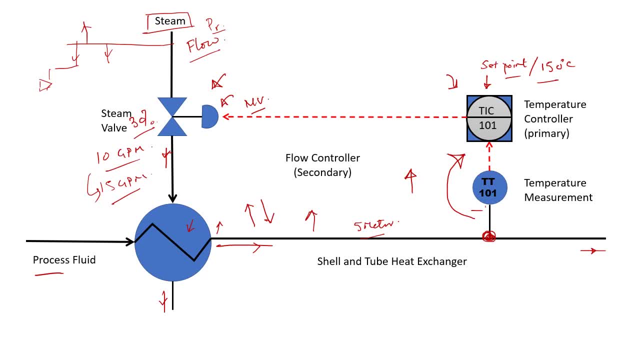 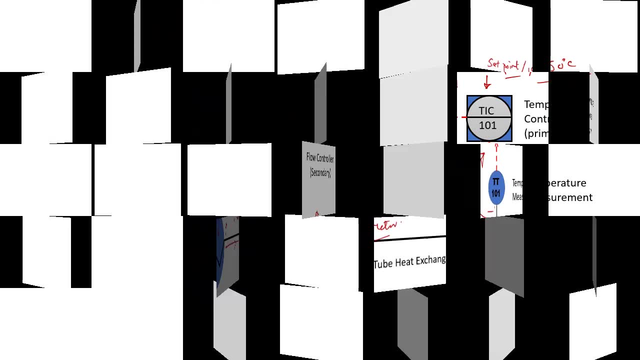 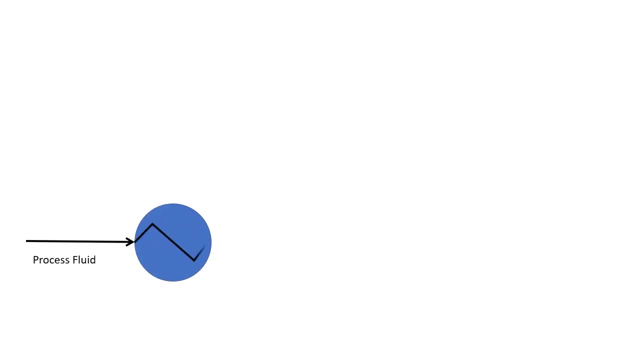 we need to control and how we will control this thing. so imagine this situation where you have, yeah, now imagine the same thing, same thing, everything is same, like the earlier case. only change is a, instead of waiting for the temperature to increase and the temperature controller to respond. 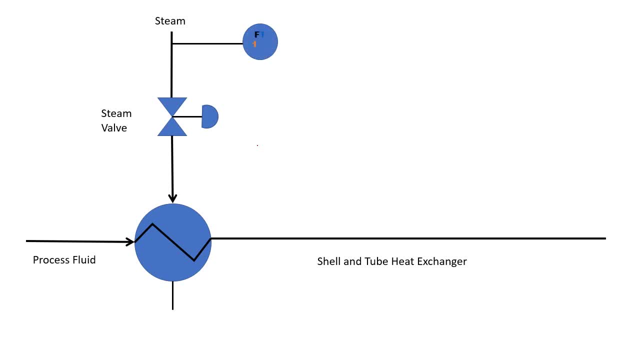 we can have another flow transmitter on the upstream of the steam valve which will sense the change in the flow and ask the steam valve to open or close accordingly, and this particular controller will will get set point from the output of the temperature controller. right so the output of the temperature controller. 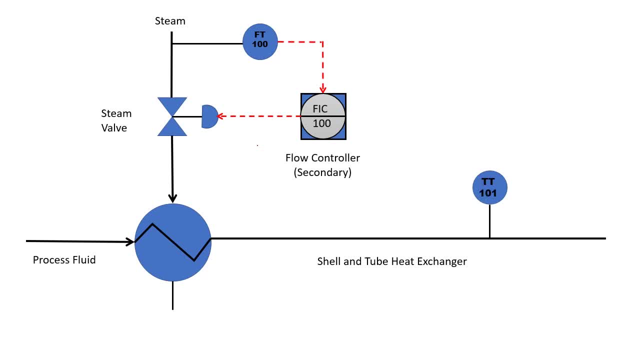 ah, will be the set point of this flow controller. so so now we have two controller: one is temperature controller and another is flow controller. The temperature controller is known as the primary controller, as this is the primary variable, or temperature is the primary variable that we want to control, and the flow controller 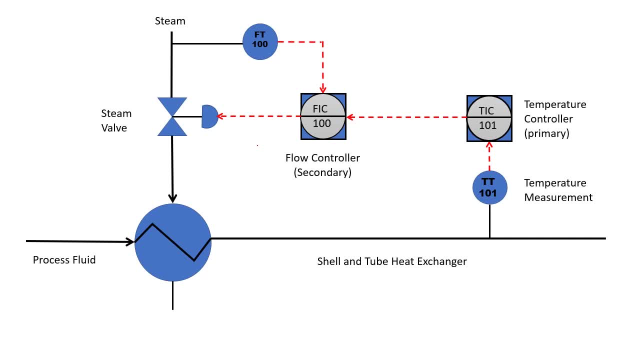 is a secondary controller right. So the output of the primary controller, this MV, becomes the set point for this controller. okay, So operator like other case operator will give set point here. So this is the operator. set point will come here. 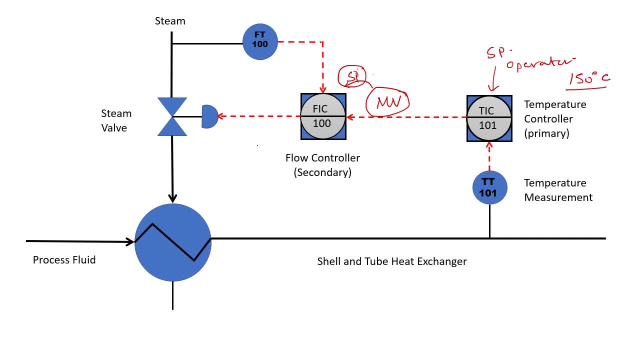 So it is the same thing. It will be like operator set point is giving 150 degree centigrade. So the temperature will be sensed: temperature controller. based on the algorithm, it will generate the MV and this MV will be the set point of the flow controller. 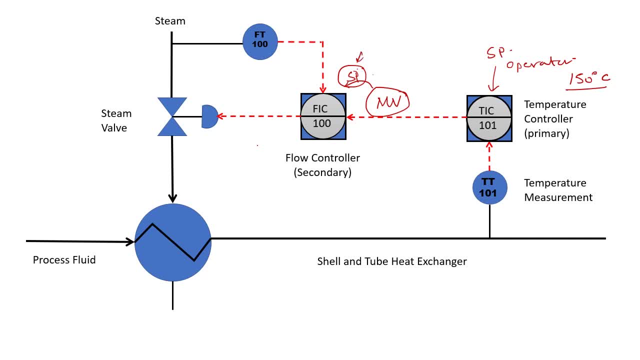 Flow controller will see this set point and also the flow Measurement it will see, and then it will be providing output to the steam valve. If there is no disturbance in this flow line, if this flow is like becoming steady, then you can say that temperature controller is like directly driving this flow controller. 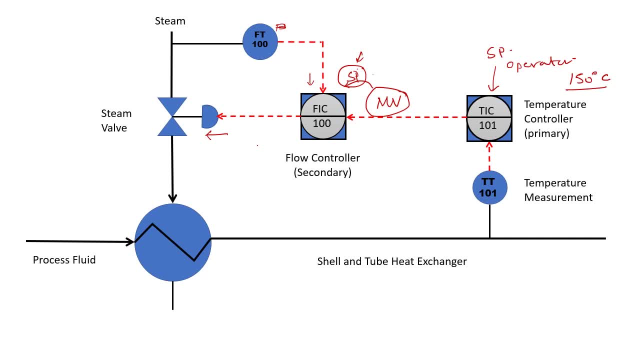 right. So only thing that happens here is if there is a sudden disturbance in the steam, then that can be used Immediately read by the secondary controller and it will take immediate action. It will not wait for the temperature to change and then change the steam valve output, right. 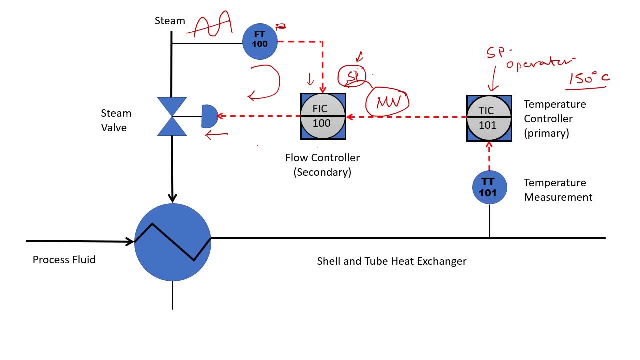 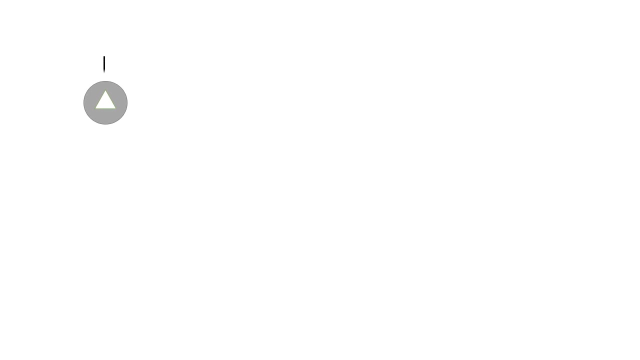 So this is the immediate action and this action will help in stabilizing your process, to more accurately control your process and without disturbing your downstream things. right, So this is The concept of the cascade control. Now, if you, if we want to show in a schematic manner which normal textbooks provide, 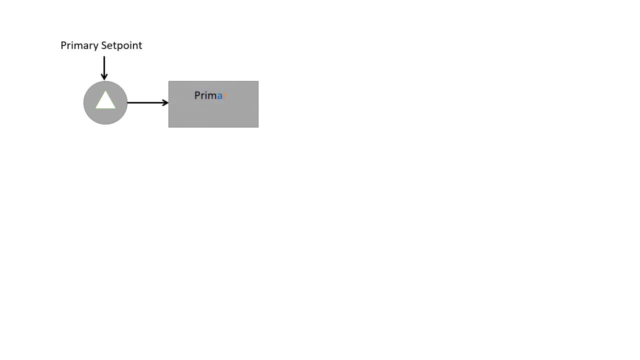 So this is this is the. this is the schematic. As you can see, there is a primary controller. The primary controller is getting set point from the operator and it is giving Output to the secondary controller Right, And the secondary controller has another sensor that is coming into it. 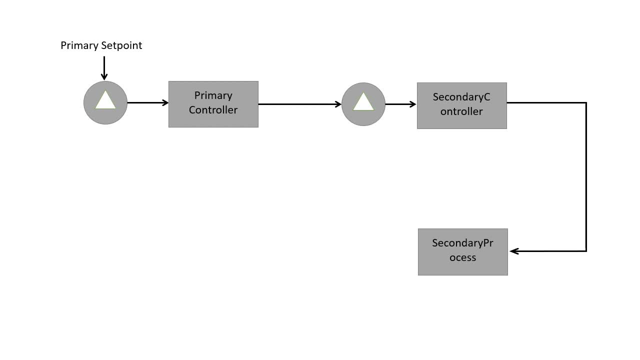 Okay, And the secondary controller provides and secondary output goes to the secondary process- Yeah, And then it goes to the primary process. So secondary process in this case is obviously the flow. primary process is your temperature. so this is the whole casket. 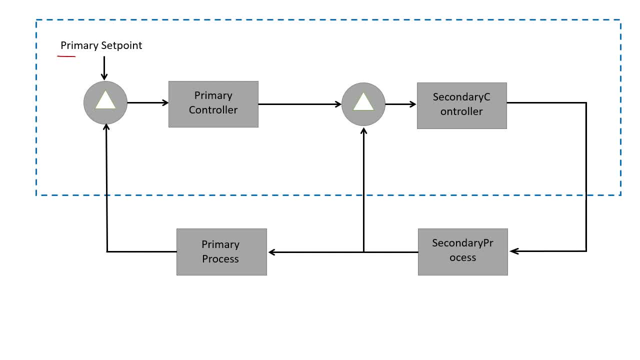 loop, if you can see. so this is the primary set point. that operator keeps right and this goes into the primary controller and it takes the input or feedback from the primary process, which in this case is the temperature, and then this output, this MV, becomes, actually, becomes set point for this controller. 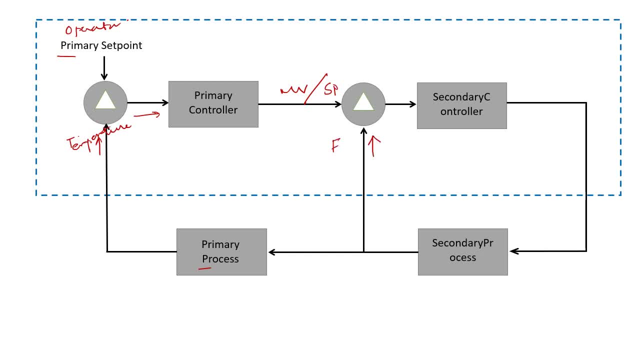 and this is the process- input from the secondary so, which in this case is flow. so, based on this set point and flow, it will generate our output that will go into the secondary controller and it will go to the secondary process then. so this is the normal schematic of a cascade control system. 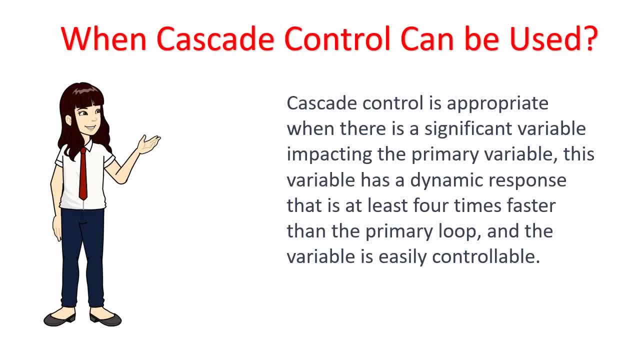 now when the cascade control can be used, whether we can use in every cases, or what is the parameter that needs to be fulfilled for implementing a cascade control. so one of the thing is so we should have like there is a significant variable, so in this case the flow is a significant variable right which can 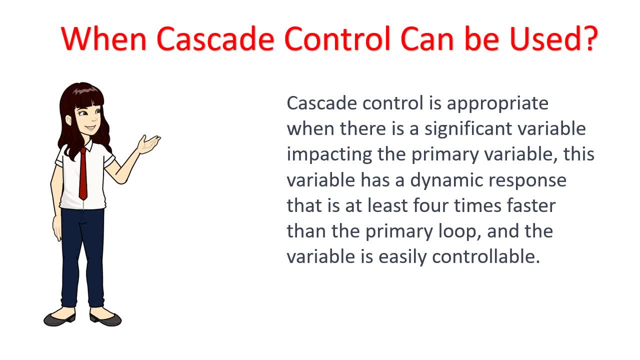 affect your primary variable, which is temperature. so this is the flow, is your secondary variable and it has the potential to vary the temperature, right? so this relationship should be there. so suppose, instead of flow, if we take any other parameter, say, maybe instead of flow would take maybe the composition right? 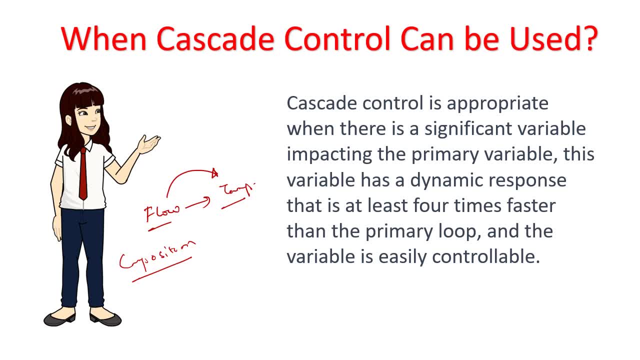 composition of the steam, whether it has effect on temperature. maybe it has, but maybe the effect is very minimal or the relationship is not very clear, right? so in that case this composition cannot be a secondary variable right. second is the secondary variable dynamics. response should be at least four times faster. 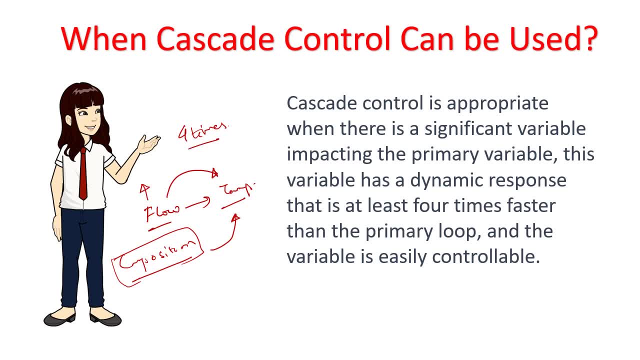 than the primary one. so in this case flow reacts much more first compared to the temperature. so temperature same changes in a slow manner, right so? so that is another thing. so dynamic response should be faster and the variable should be easily controllable. in this case we can easily control the. 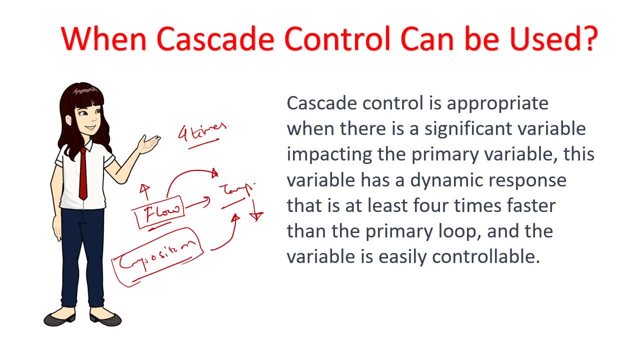 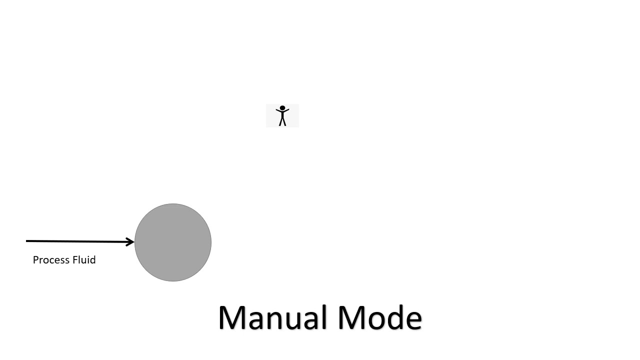 flow with the help of a control valve right and a flow sensor. so if it is some other parameter, say for like composition, controlling the composition and measuring the composition is very difficult task, right, so it cannot be used as a secondary variable. now there are basically different modes in which the cascade control loop can be operated. 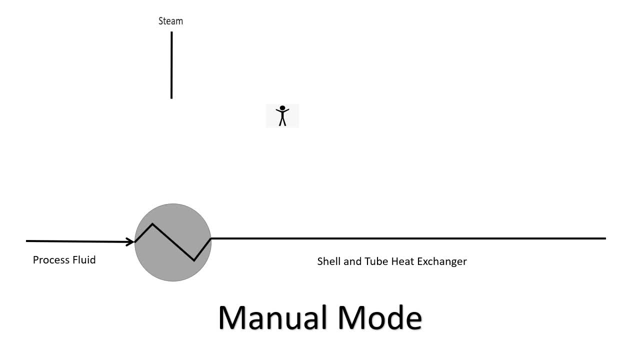 for example, the example we are taking of the heat exchanger, it may happen that you want to keep your secondary loop into manual. the operator wants to manually control the steam bulb, maybe during the startup operation, right? so maybe during the startup operation there is some requirement to control the. 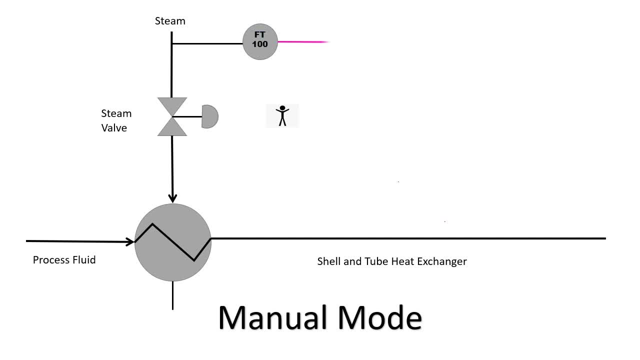 process manually. so in that case operator will take this particular secondary loop into manual. so when secondary loop is taken into manual, so operator can directly control the steam valve and in this case the secondary set point basically tracks the secondary measurement and part primary output tracks the secondary set point. okay, what set point tracking is we? 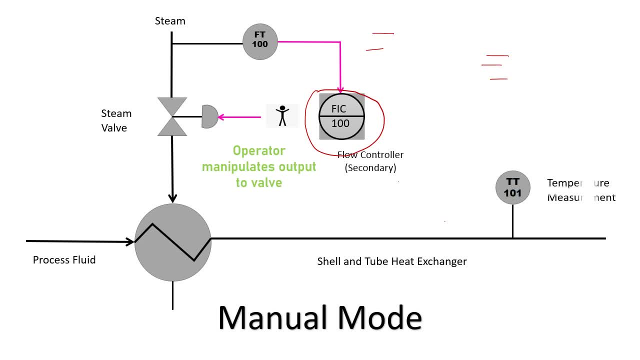 have discussed earlier, so that you can understand from other lectures. okay, set point tracking is there. so basically it is tracking the set point output, will track or follow the set point so that when this operator changes this mode from auto to manual- so sorry, manual to auto- then there will be no problem, right? so yeah, so this is the manual mode of the operation of this. 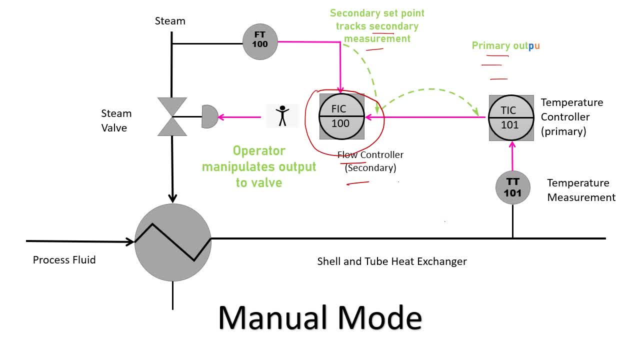 cascade controller or this flow controller. so these options are inbuilt in normal digital controller or dcs. you just need to change it from auto to manual and, yeah, it will definitely work. so there are basically, if you see normal dcs, there are three modes: one is auto, one is an manual and another is cascade. right, so these are basically three modes. 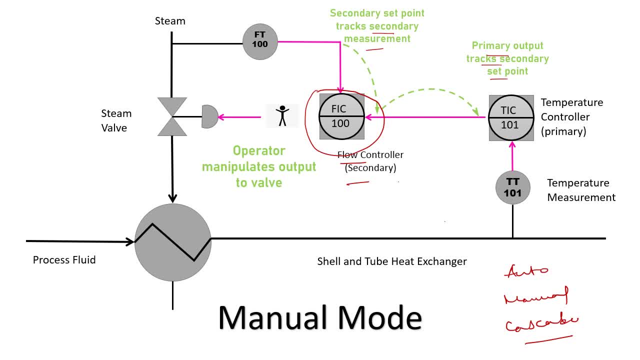 for operation in case of the cascade controller, and there is another mode which is, like, known as prd. uh, what happens in that case is: uh, in case your this ft is not reading correct, right, so you don't want this input to uh act on this. so, in that case, this, basically this tt and this. 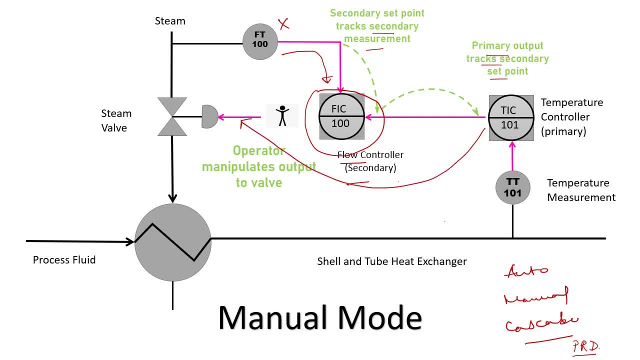 temperature controller directly drives this output right. so in that case we are bypassing this secondary loop counter completely and directly. the temperature controls the steam valve like a normal feedback control loop, so that is known as the prd. now we have discussed about this manual and prd next go into the 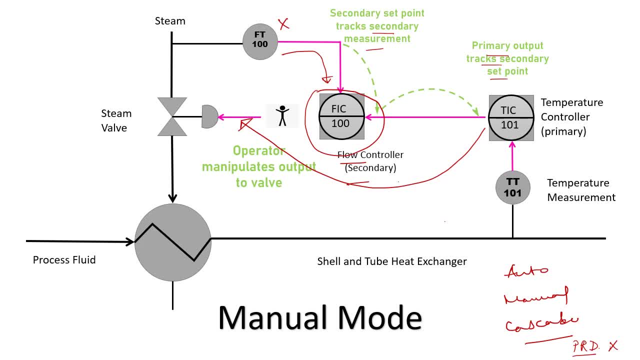 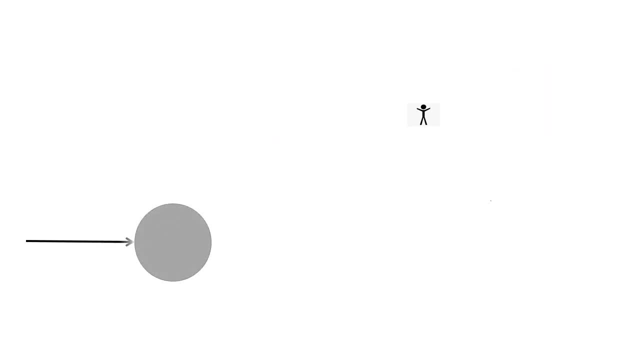 other two option, which is cascade and auto, and additionally, Sylvia also offered a Fixingimport review autofocus ınd. this is not possible. cact leaf contrast crisis at the moving speed equal or爱من right. so this is basically the auto mode. and now what is the cascade mode? cascade mode is what we. 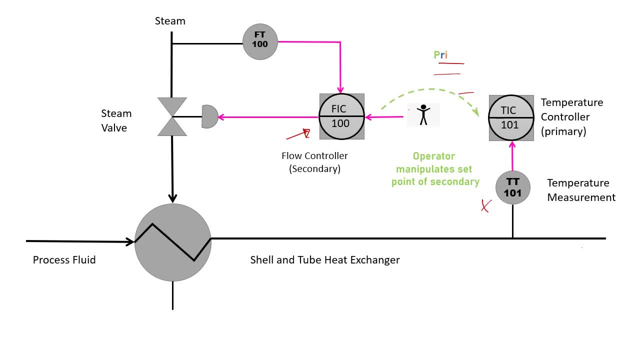 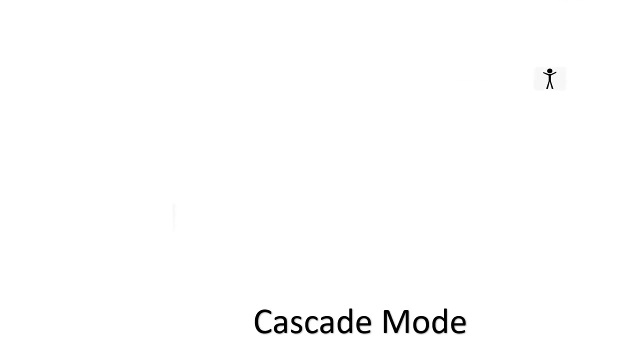 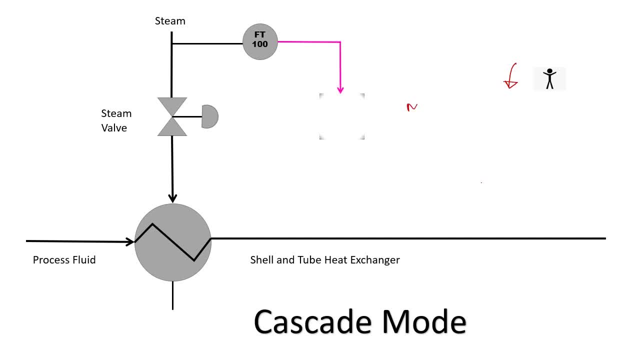 it is like operator gives a set. it is like operator gives a set point to this primary controller and primary point to this primary controller and primary point to this primary controller and primary controller. MB goes as a set point controller. MB goes as a set point controller. MB goes as a set point to set point to the flow controller. right. 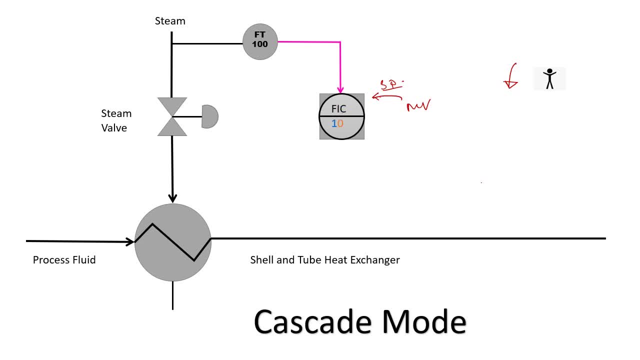 to set point to the flow controller right. to set point to the flow controller right. so this is like normal mode of operation. so this is like normal mode of operation. so this is like normal mode of operation, normal mode of cascade operation. when. normal mode of cascade operation when. 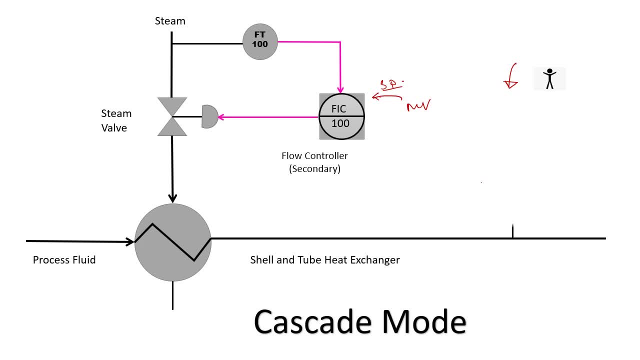 normal mode of cascade operation when everything is healthy, the temperature, everything is healthy, the temperature, everything is healthy. the temperature transmitter flow transmitter. everything is transmitter flow transmitter, everything is transmitter flow transmitter. everything is healthy and there is no issue with any. healthy and there is no issue with any. 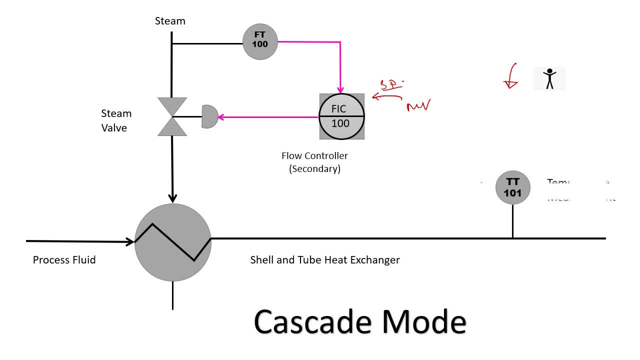 healthy and there is no issue with any of these things, right, so, yeah, so one of of these things, right so, yeah, so one of of these things, right so, yeah. so one of the major issues, as we normally find the major issues, as we normally find the major issues as we normally find, with the cascade control is 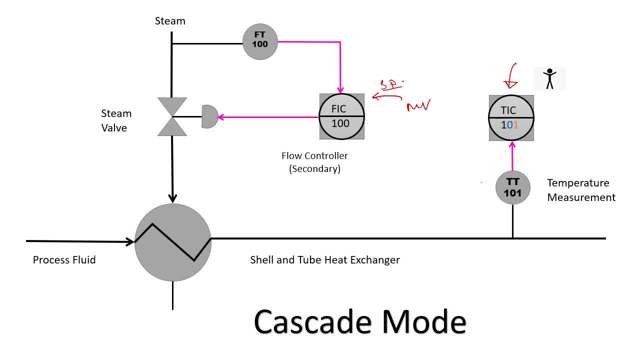 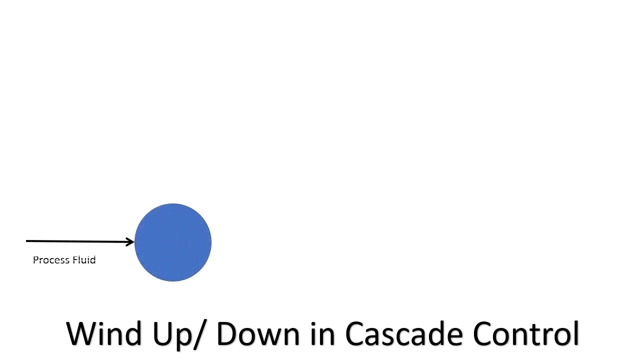 with the cascade control is with the cascade control is wind up and wind down. so what is wind up, wind up and wind down? so what is wind up, wind up and wind down? so what is wind up and wind down? we have discussed with and wind down, we have discussed with. 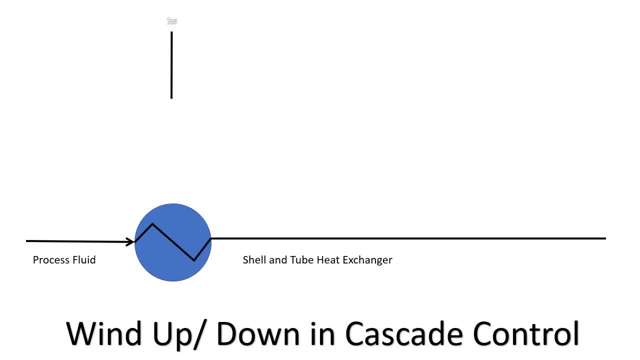 and wind down, we have discussed with respect to the integral control and respect to the integral control and respect to the integral control and there and it has been discussed, I will there and it has been discussed, I will there and it has been discussed. I will provide the link in the description box. 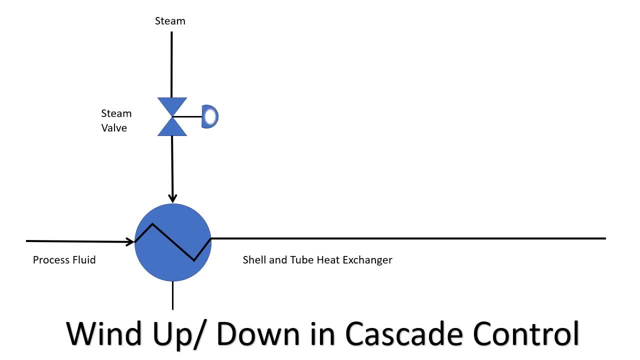 provide the link in the description box. provide the link in the description box also if it is required. so what happens also if it is required? so what happens also if it is required. so what happens in this case is basically basically if. in this case is basically basically if. 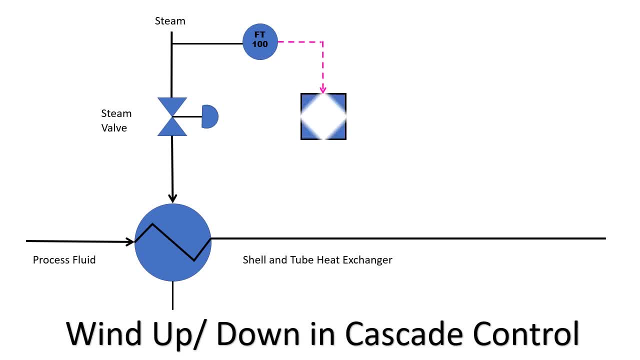 in this case is basically, basically, if, like, if there is a change in the like. if there is a change in the like, if there is a change in the temperature of the steam right, so due to temperature of the steam right, so due to temperature of the steam right, so due to any disturbance of the upstream process. 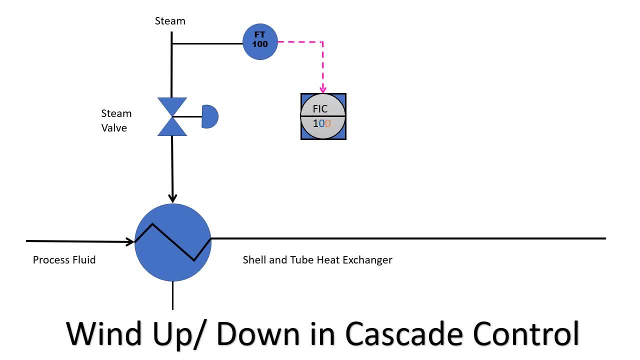 any disturbance of the upstream process, any disturbance of the upstream process, right, right, right. so in that case, what will happen? so it will. so, in that case, what will happen? so it will. so in that case, what will happen? so it will happen that the process fluid, happen that the process fluid. 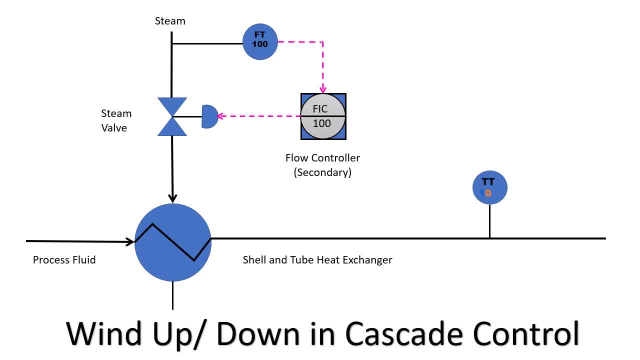 happen that the process fluid temperature goes below the setpoint right, temperature goes below the setpoint right. temperature goes below the setpoint right, the required setpoint is not meeting, the required setpoint is not meeting, the required setpoint is not meeting and in that time the temperature 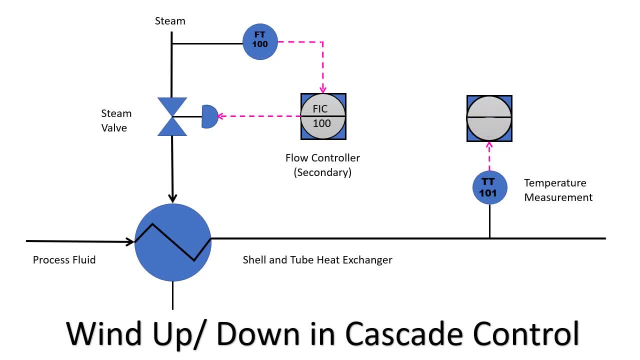 and in that time the temperature and in that time the temperature controller will drive the flow controller will drive the flow controller will drive the flow controller for further opening of the controller, for further opening of the controller, for further opening of the steam valve and, and it will know if, 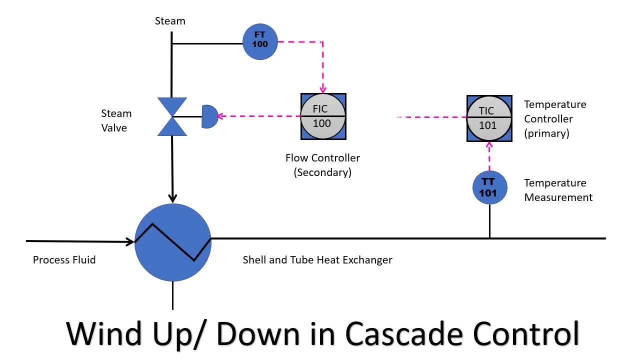 steam valve and and it will know if steam valve and and it will know if it will increase its setpoint until until it will increase its setpoint, until until it will increase its setpoint until until the temperature is met and if the the temperature is met and if the 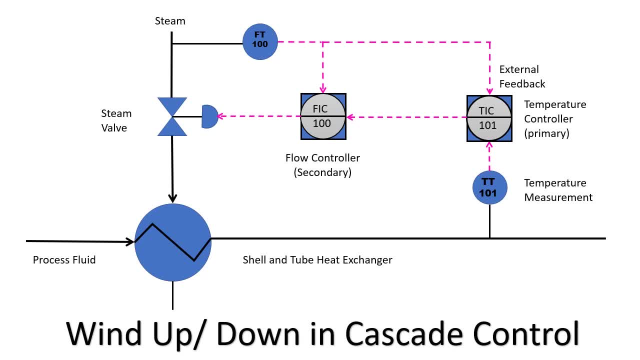 the temperature is met and if the temperature is not met, it will increase. temperature is not met, it will increase. temperature is not met, it will increase to such a level that the steam valve to such a level, that the steam valve to such a level that the steam valve opens fully. right now, if that steam 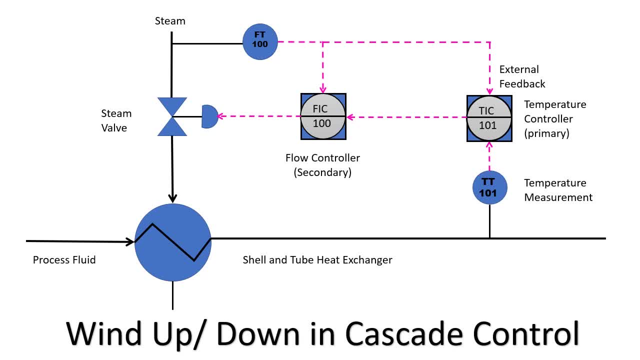 opens fully right now, if that steam opens fully right now, if that steam temperature again becomes normal, then you temperature again becomes normal, then you temperature again becomes normal, then you, you have to come down from the hundred. you have to come down from the hundred, you have to come down from the hundred percent open stage to the below stage. 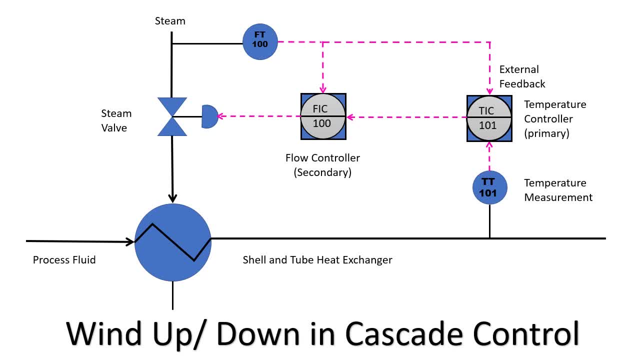 percent open stage to the below stage. percent open stage to the below stage: right. so this is in this case, in this right. so this is in this case, in this right. so this is in this case, in this case. wind down sometime takes more time. case: wind down sometime takes more time. 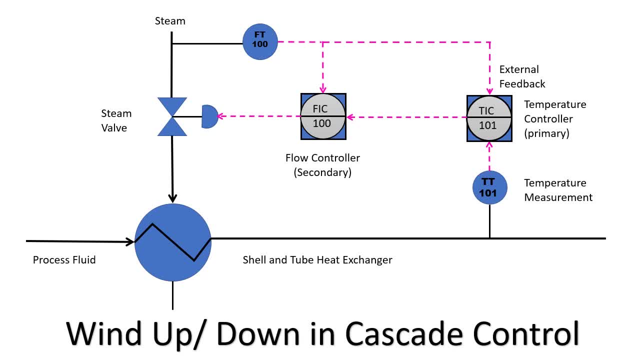 case, wind down sometime takes more time right, and that causes the upset in the right and that causes the upset in the right and that causes the upset in the process. so how to avoid this is to by process. so how to avoid this is to by process. so how to avoid this is to by means of providing external feedback. so 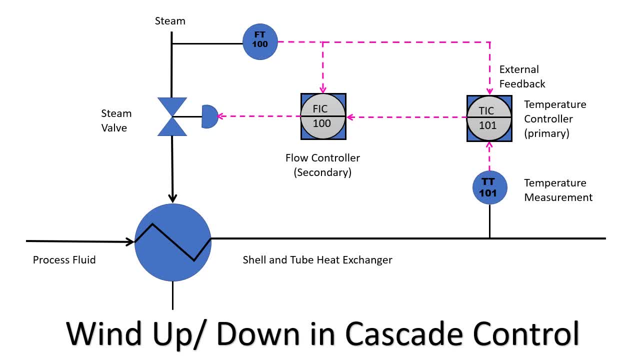 means of providing external feedback. so, means of providing external feedback. so now the flow input will go directly to now. the flow input will go directly to now. the flow input will go directly to the temperature controller and it will the temperature controller and it will the temperature controller and it will help in resetting the controller right.